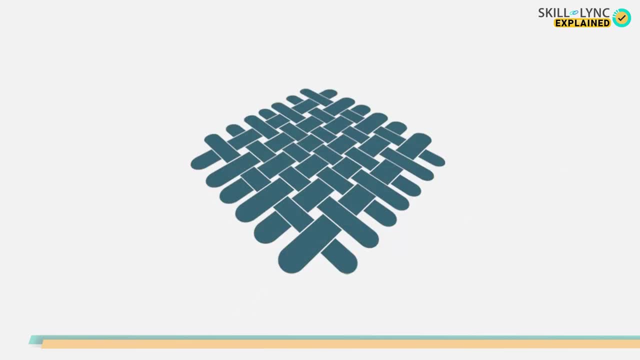 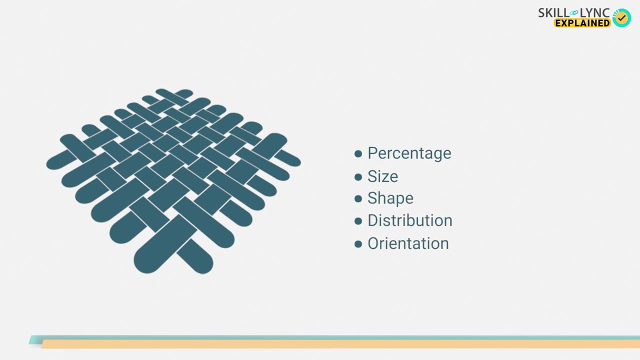 dispersion phase. The properties of the composites vary according to the percentage size, shape, distribution and orientation of the dispersed phase in the matrix phase. When it comes to classification, composites are of three different types. They are particle reinforced composites, fiber reinforced composites and structural composites. Let's discuss. 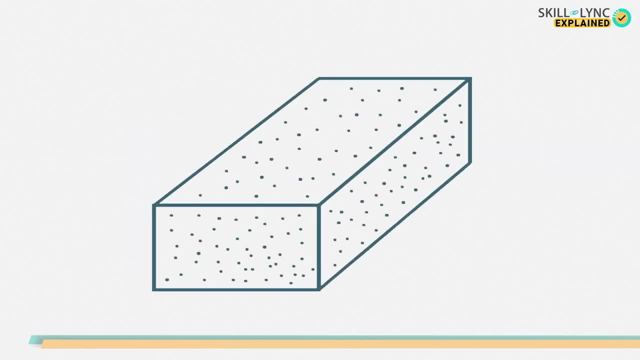 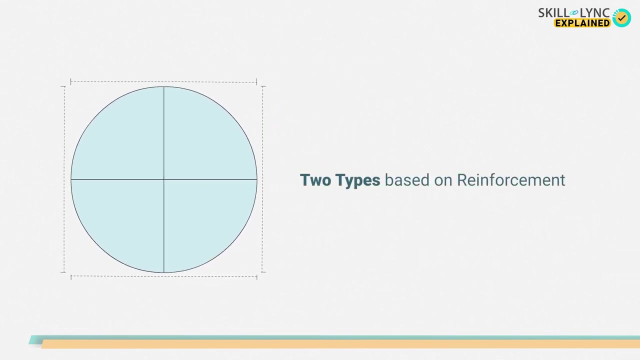 all these types one by one. Particle reinforced composite is a type of composite that uses tiny particles as its dispersed phase. These particles are characterized by their equal dimensions in all directions. These particle reinforced composites are further classified into two types based on the reinforcement mechanism. 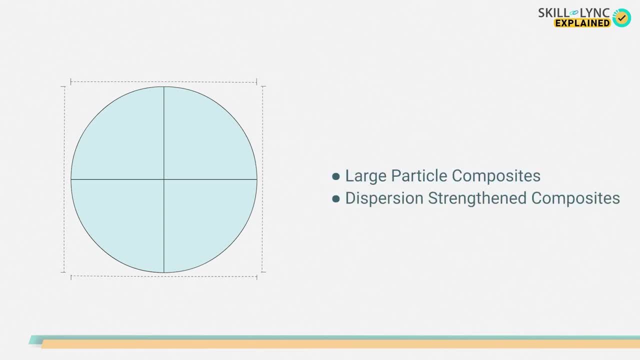 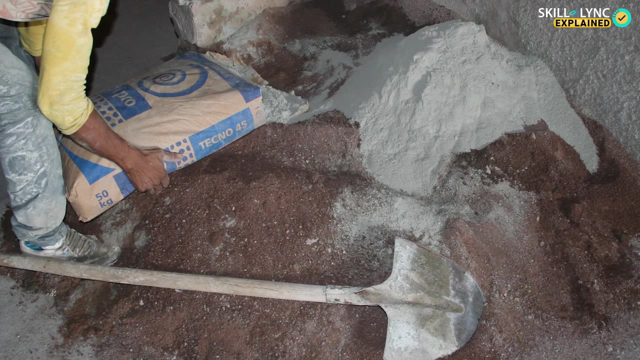 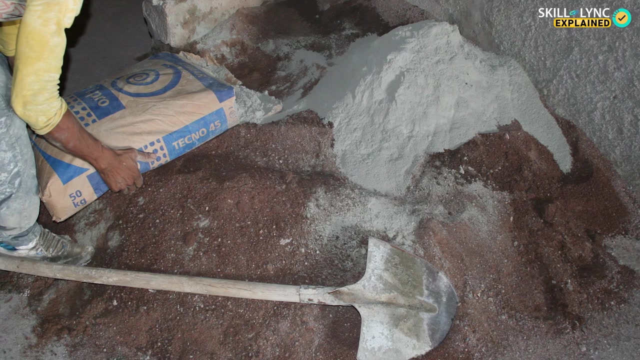 They are large particle composites and dispersion strengthened composites. In large particle composites, the interaction between the phases should be treated at the continuum level. If you don't know what continuum is, check out the link in the description below. Here, the filler material replaces some volume of the material and modifies its property. 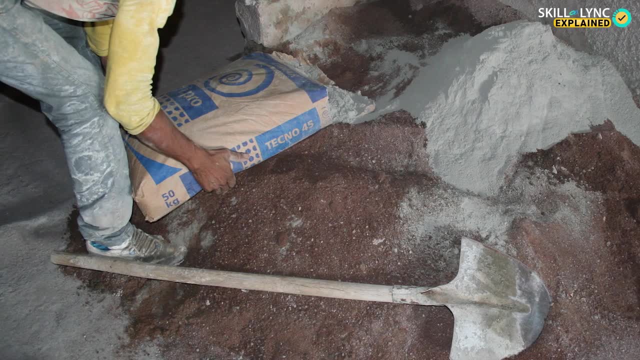 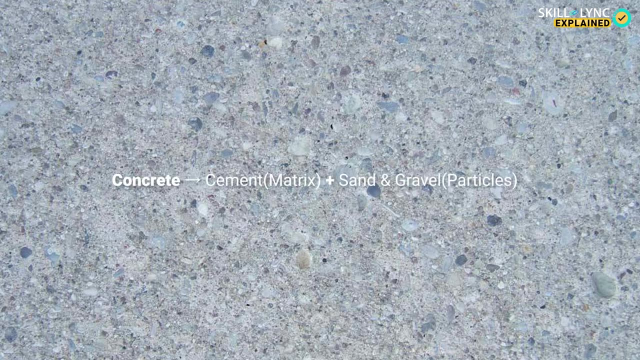 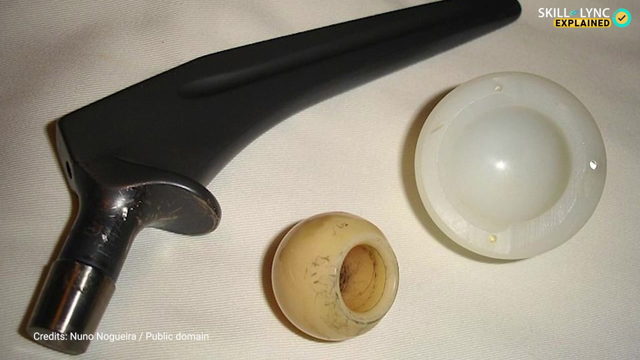 The change in property depends on the volume of the filler material. Concrete is a very good example of this type. Here, cement acts as the matrix, and sand and gravel acts as the particles. Another example of this type is ceramics, which are the composites. 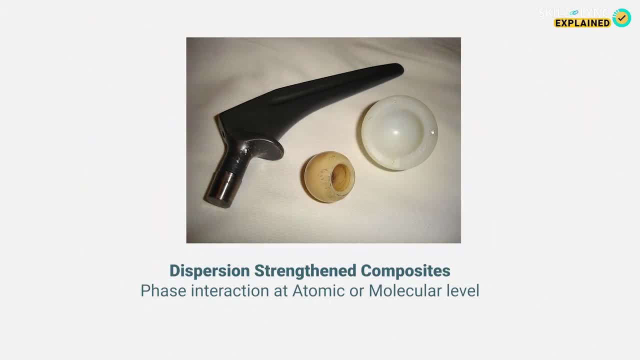 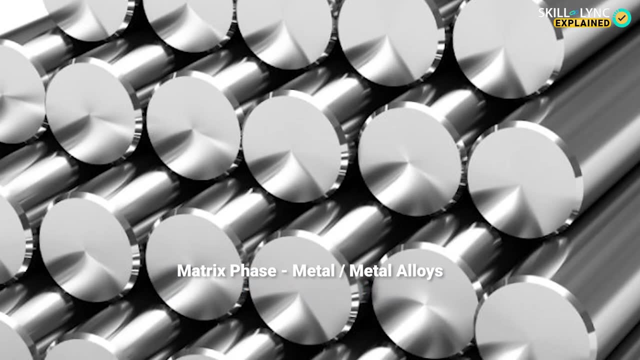 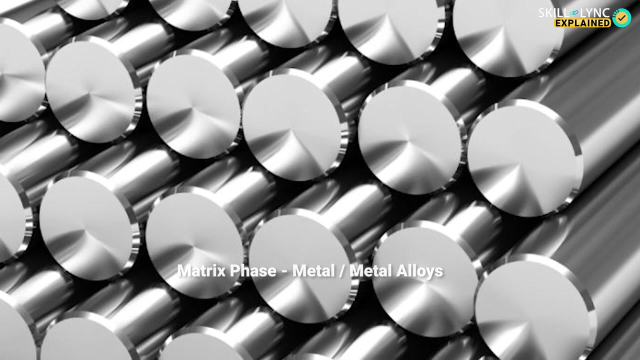 made of ceramics and metals. When it comes to dispersion strengthened composites, the phase interaction takes place at the atomic or molecular level. Here a certain volume of fine material is added to a hard or strong material like metals and metal alloys. The dispersed phase can either be metal or non-metal. 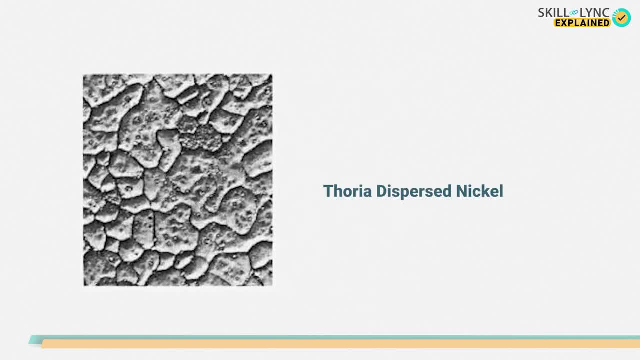 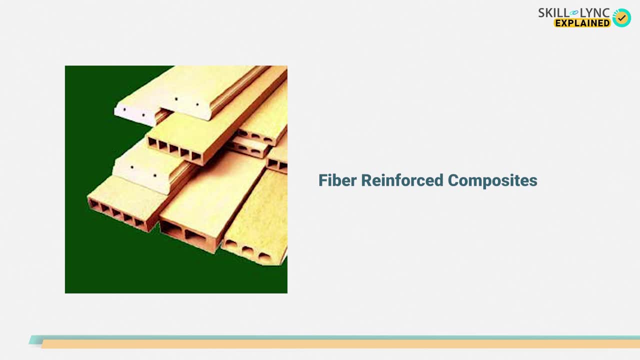 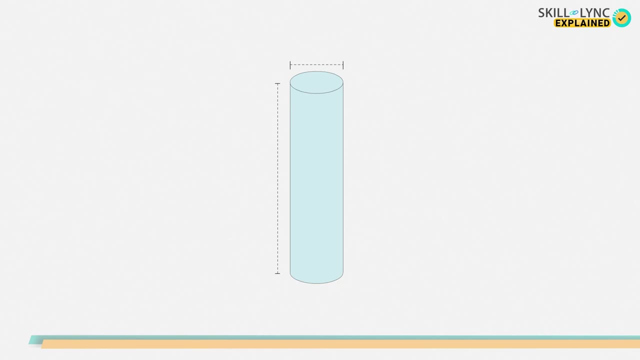 An example for this type of composite is Thorium dispersed nickel. It's a type of nickel alloy that has 3% of thorium in it. The next type of composite is the fiber reinforced composites. Fibers are characterized by their length to diameter ratio. They possess high strength.